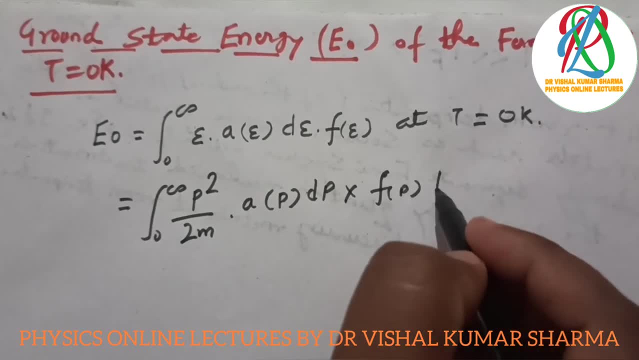 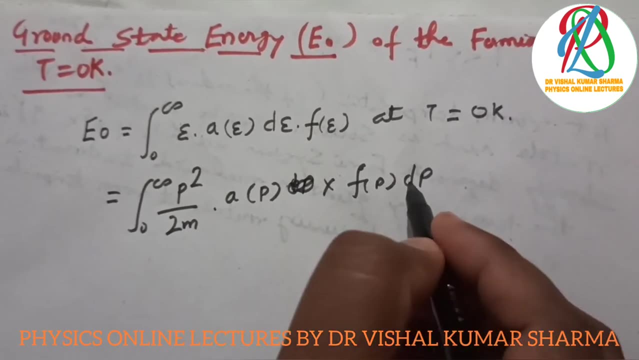 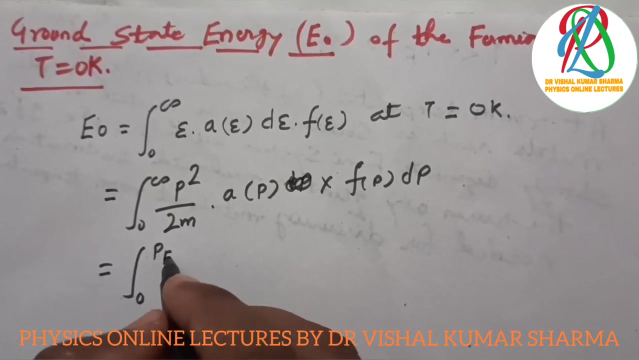 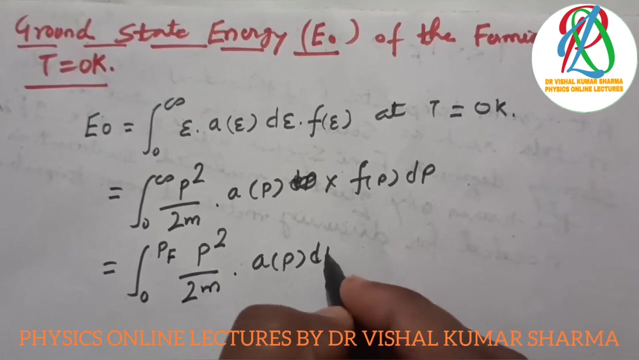 dp here into this f of p, dp here. So from here you can just write, from here this: this is here dp, so we can have this 0, 2. now the limits will be this: p, f. so it is here p, square upon 2 m, and it is here a p. this is dp, and you know that when we are discussions of this. 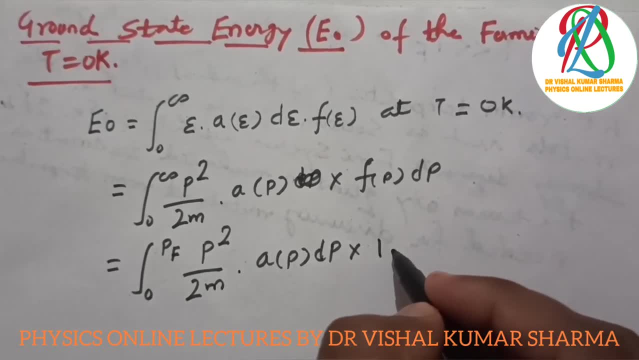 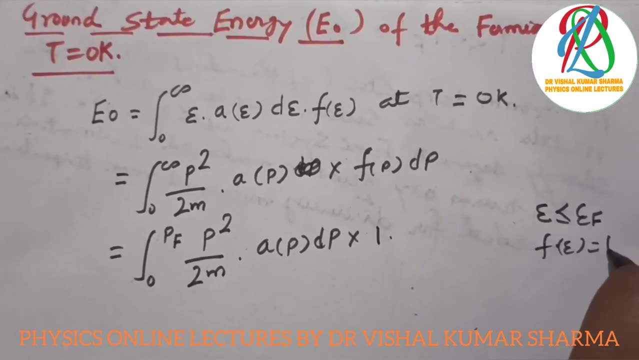 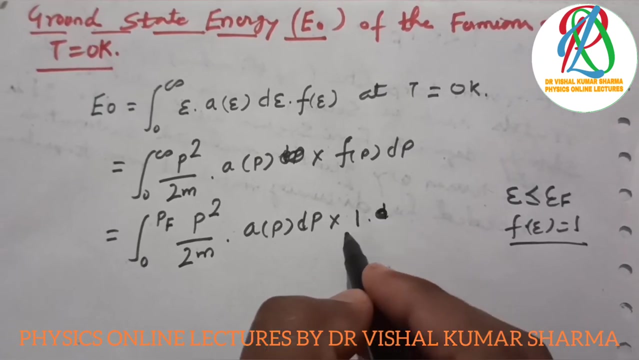 correspondence we have the distribution function is 1 when this is the condition less than equals to f, the fermi distribution function. this have the value unity here. so we have just write here this value, this in terms of either. you can just have, this is here, one here. so if we just calculate, 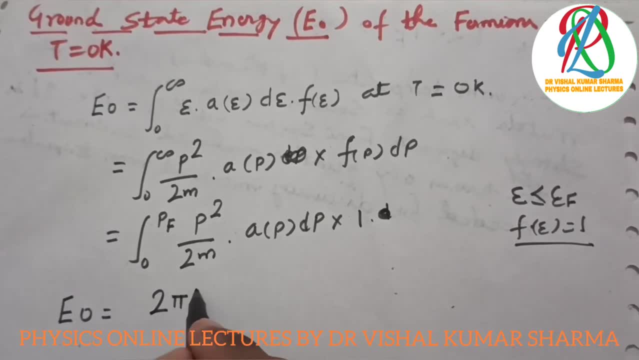 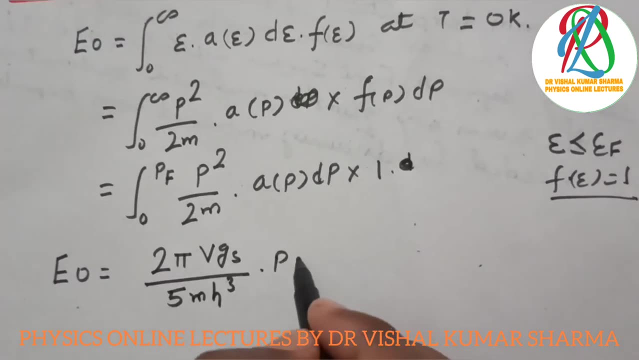 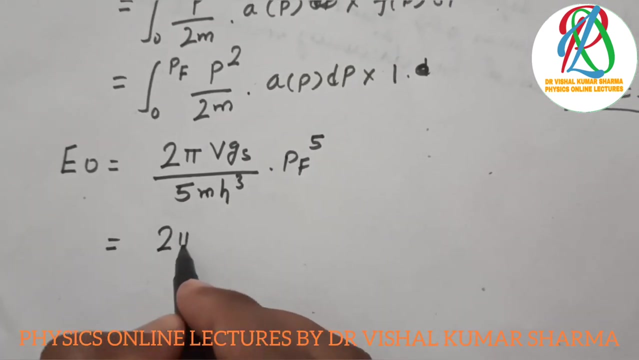 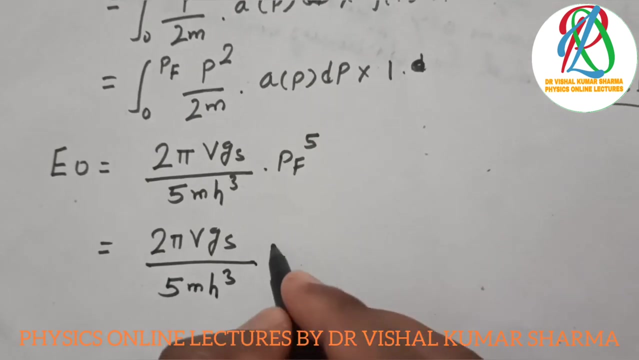 its value. it comes out to be simply 2 pi v g s upon this 5 times of m of s cube into p f to the power, this 5 here. or simply you can just say here: this is 2 pi v g s upon this 5 m of s cube here. you can just write here in terms of this momentum: 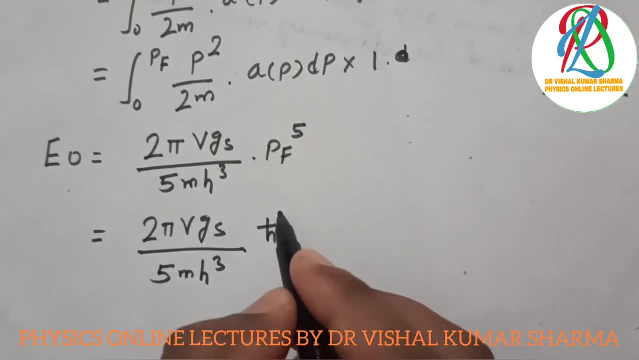 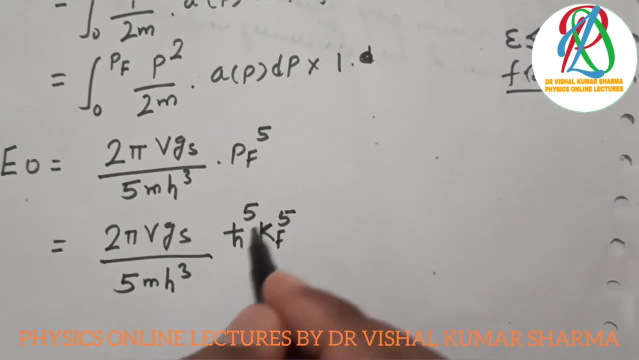 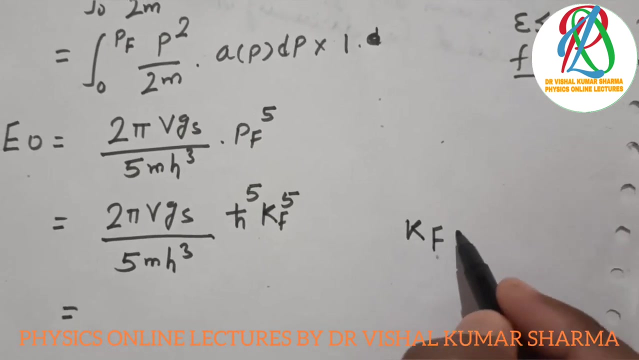 or wave vector. this fermi momentum can be written as h raised cross to the power 5, this k f to the power 5 here. or simply, if we just made some arrangements where k f this fermi vector, you can just say fermi wave vector. 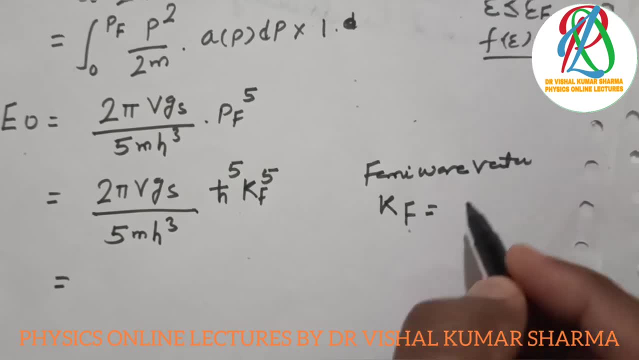 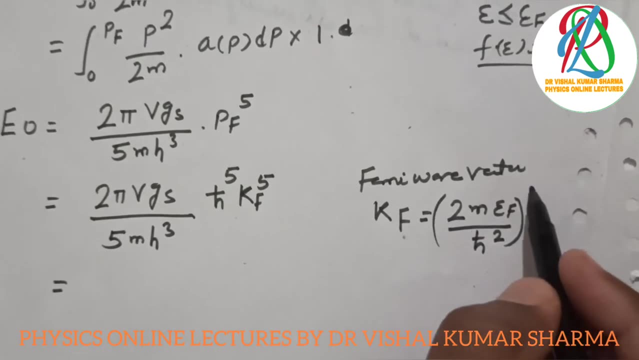 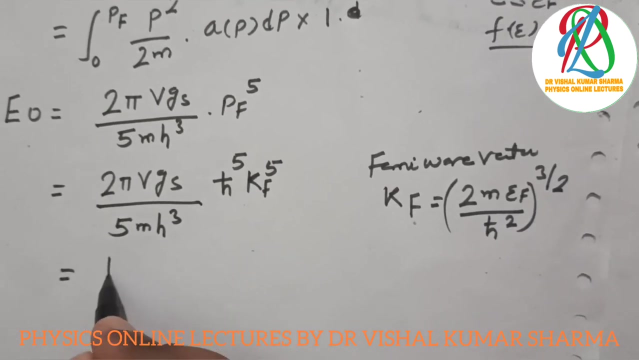 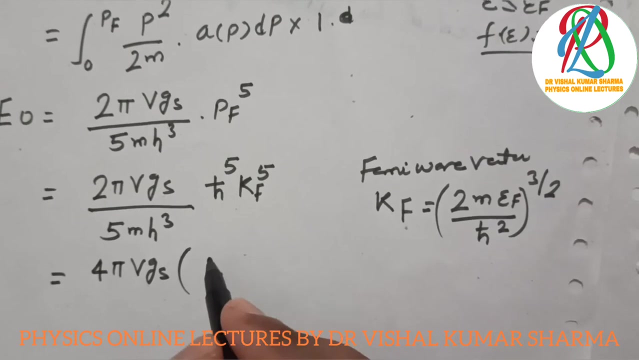 this is given by the formula. you can just say this twice: m, epsilon, f upon this h cross square to the power. this is 3 by 2 here. so from here you can just see: this is here 4, pi, v, g, s, and i am just making here the some arrangements here so you can have this h cross square, k, f square. 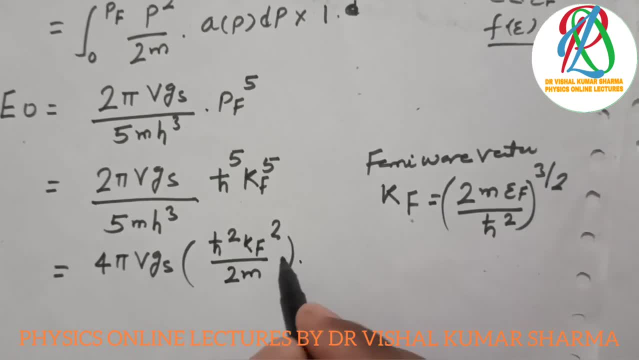 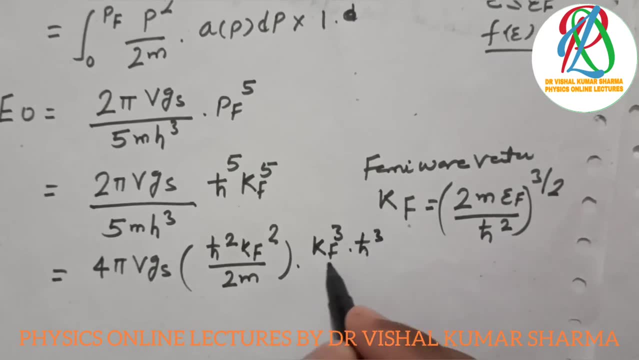 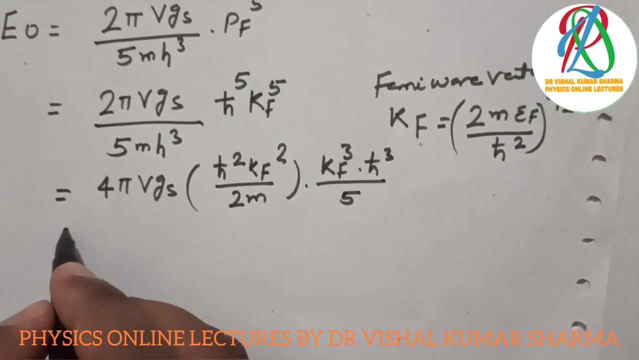 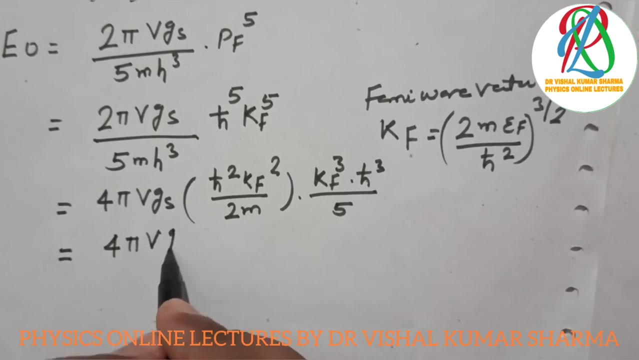 upon this twice m. and what is the remaining term here? just here, this k f cube and h cross cube. upon this: 5. here it is simply the above term. i have just written with certain rearrangements here, so if you just solve it, this comes out to be- look at here carefully: 4 pi. this is here v g s upon this. 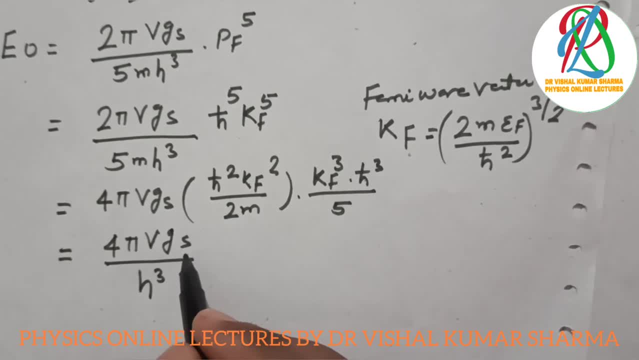 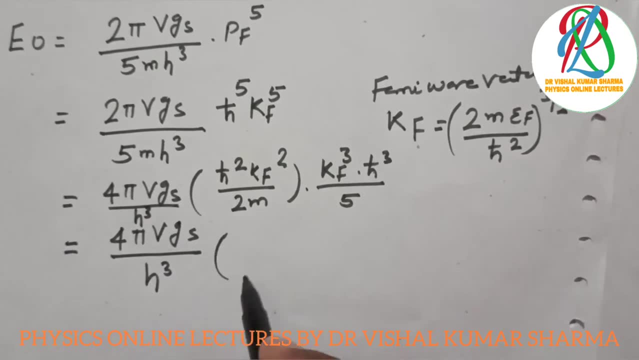 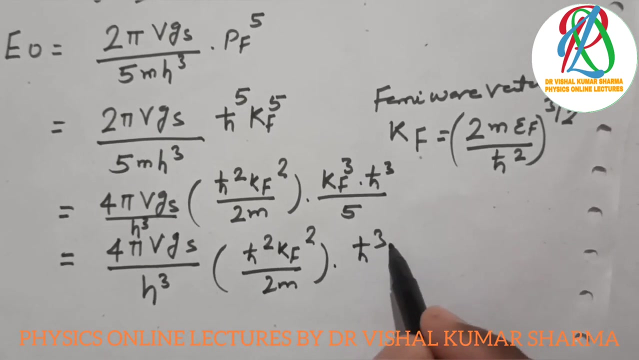 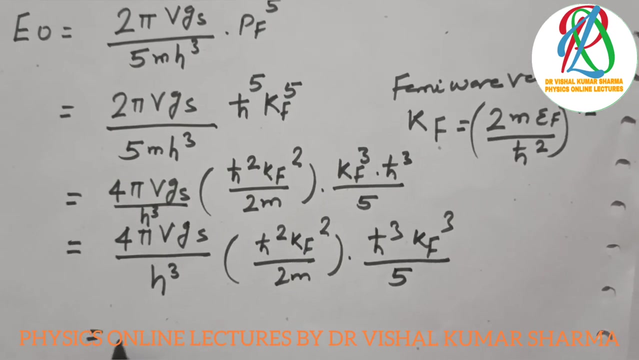 h cube. it is here, so there, it also already here. it also present here as s cube. so in this case you will have h cross square, this k f square upon this 2 m into h cross cube, k f cube upon this 5 here. so if you just write it as: 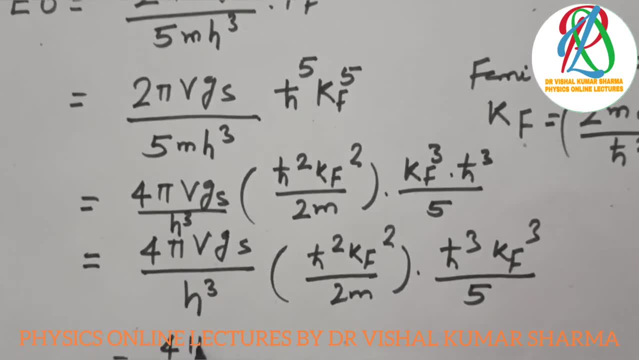 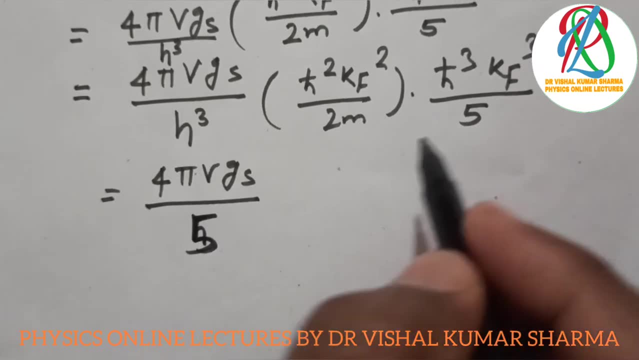 if you just solve it, you can write 4, pi, v, g, s upon this. 5 here, so'm gonna say, is equal to. so that's what we can develop in this idea here. you can just write here from this 5: and what is it? this factor just compare. 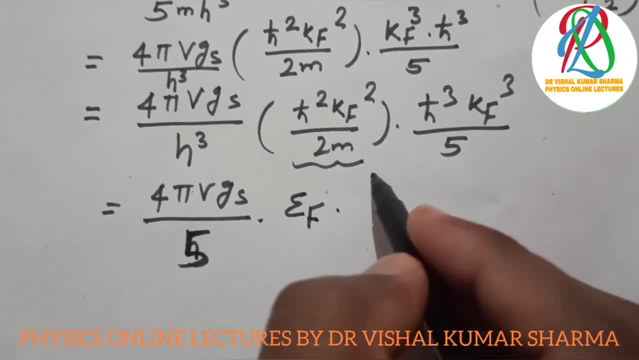 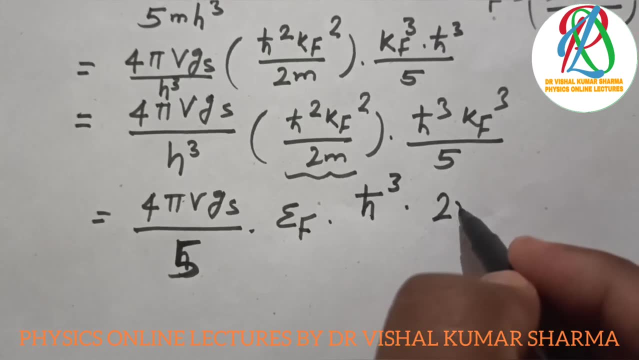 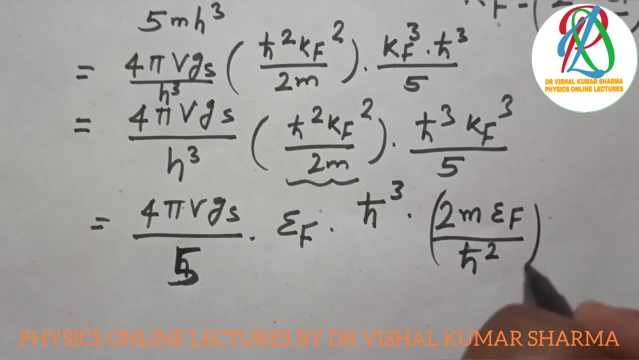 it. this is Fermi energy here, and it is here h cross Q and K F. it is here. you can, just from the above definition, this is twice M EF upon this h cross square derived with power. this is 3 by 2. so just by substituting this, if you just. 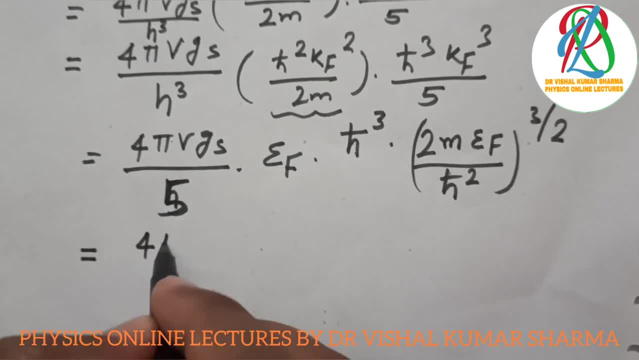 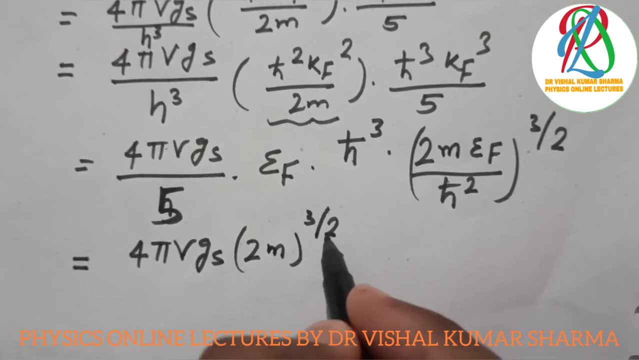 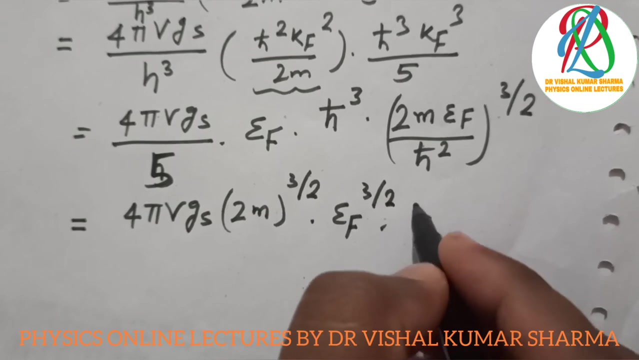 solve it. just look at here carefully. it is here 4 pi V, G s. what is here? twice M to the power? this is 3 by 2 year. what is epsilon F? it is here. you can just write 3 by 2 here, and it is you a s cross Q upon. you can just have s cube. 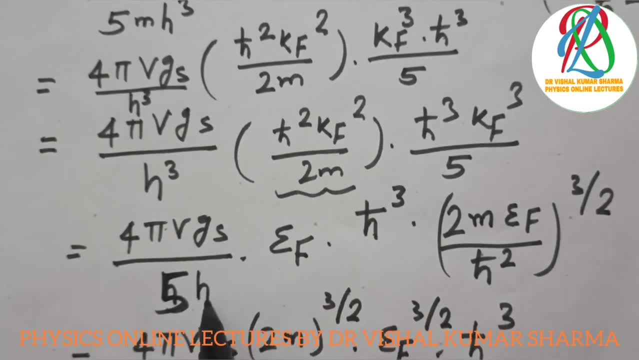 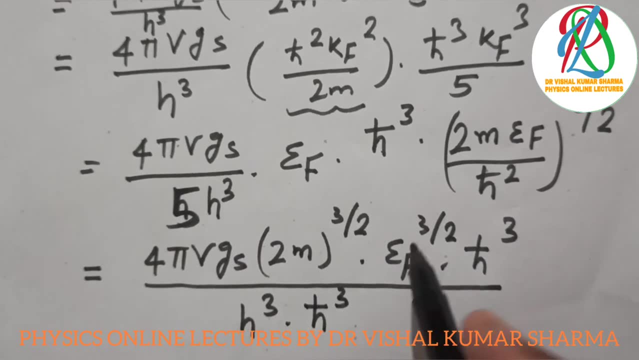 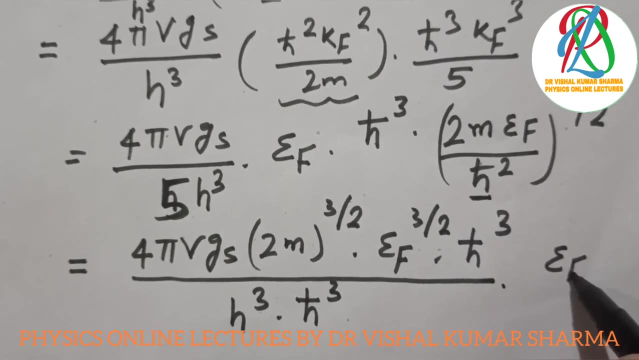 is equal to in vector 3. I think its bought these all together. and what you do to Sean? here it is already present, just here it is h cube is already present here and in this case h cross cube which is coming from, from this factor. it is h cross cube and here epsilon f. 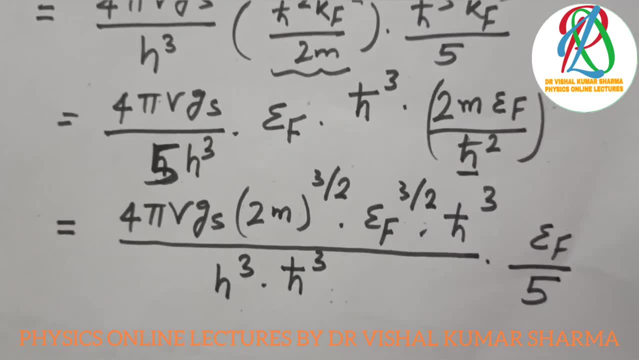 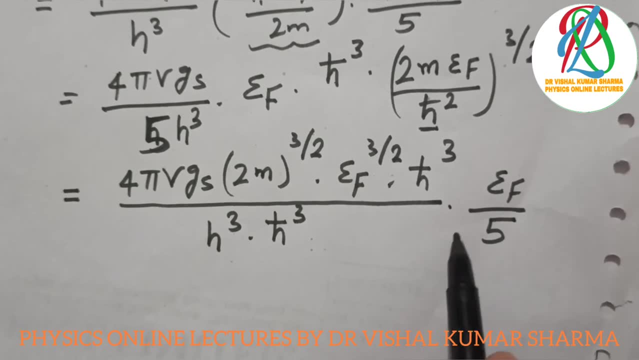 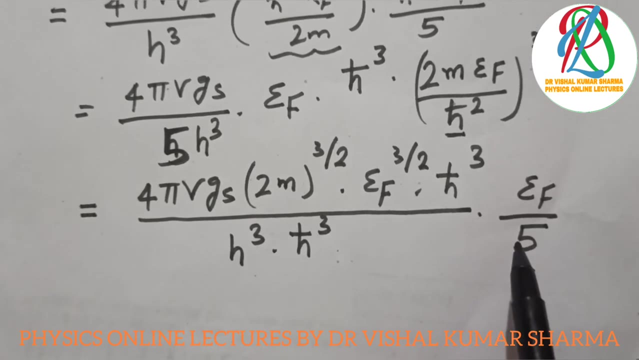 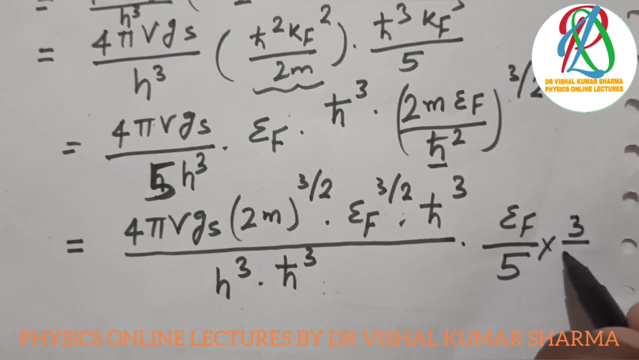 upon this 5 here. So it is just simply you can just say that if you just what we will do here, if you just multiply and divide by the factor 3 here, if you just multiply and divide by the factor 3 here, so I am just going to multiply and divide both of the factor by 3 here, so you can just see: